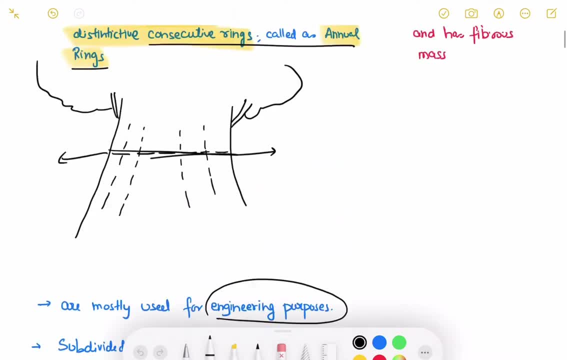 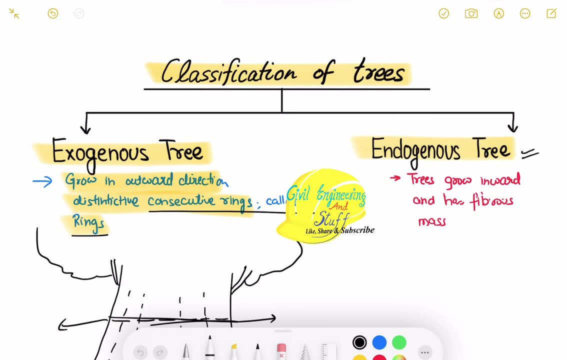 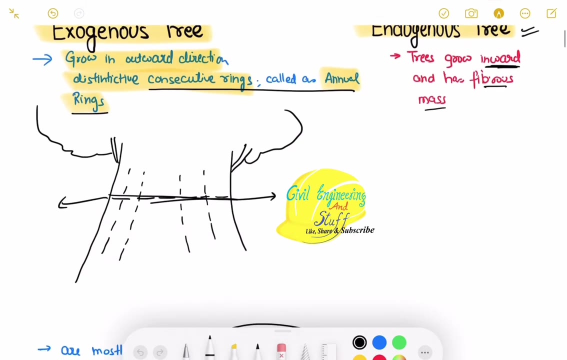 much identified from each other, Right. The second variety of trees is endogenous trees, and these trees basically grow in the inward direction. Right. These types of tree basically grow in the inward direction and have fibrous mass. so basically the growth of these type of tree happens in the inward direction, that is, they have the growth 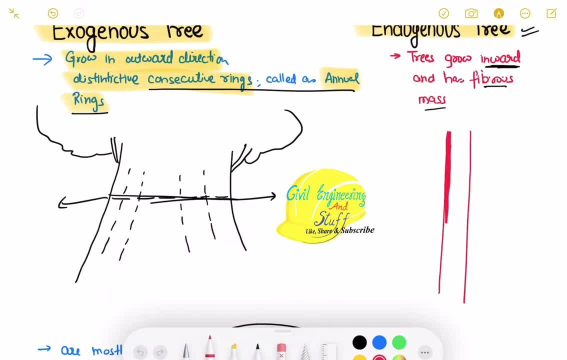 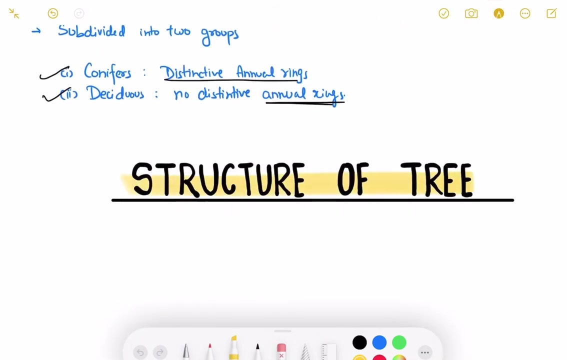 in the inward direction only, so, with time, their stem keeps on getting stronger and stronger and have fibrous mass. the example of your endogenous tree is bamboo, and your bamboos are mostly used for scaffolding purposes, right, so they use for with respect to exogenous trees is very limited. okay, then we have structure of trees, so we are going to discuss. 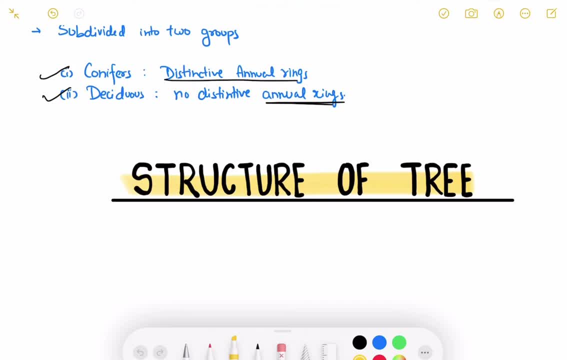 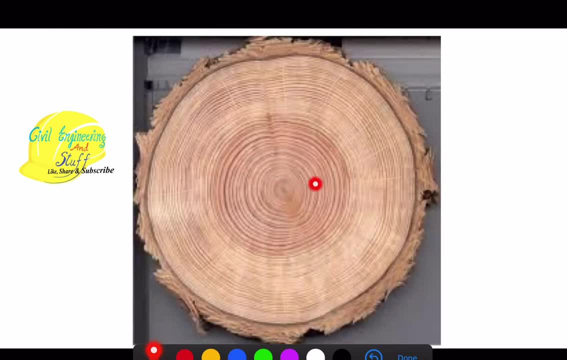 about the structure of trees or that is, of exogenous tree. so the structure of tree looks something like this: it has a central mass right around it. we have number of rings, closely packed rings right, and you can see they are somewhat darker in color. right after this there are some outer rings. 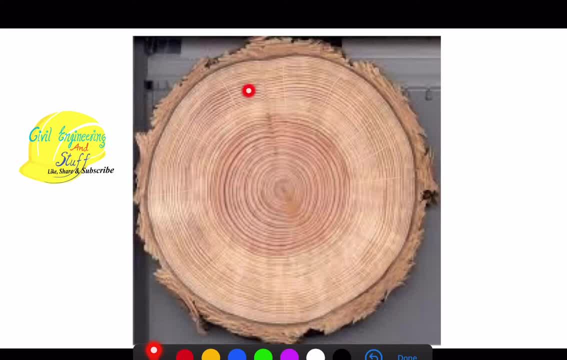 and the. with comparison to the inner rings, their complexion is somewhat brighter. right, they have light colors compared to that of inner rings. then you have the certain fibrous mass right, or sap, and after this you have bar right and you also have the radial rays that emerge from the center to the outer rings. right, 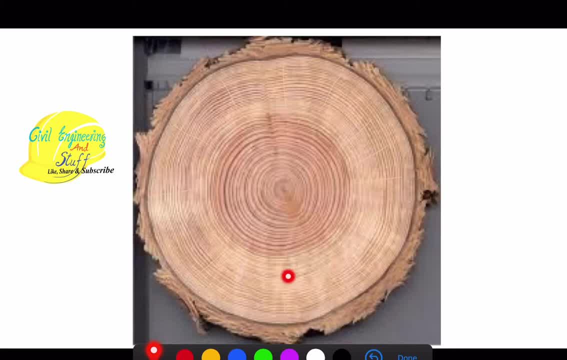 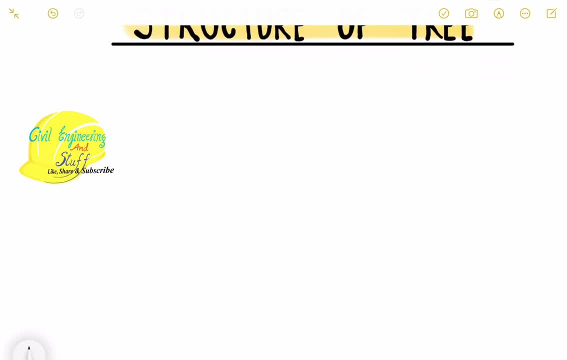 so this is how the structure of a exogenous tree looks like. so let us draw the structure of tree so, as we have seen in the figure, it has center mass and around the center mass we have number of rings. right around the center mass we have number of closely. 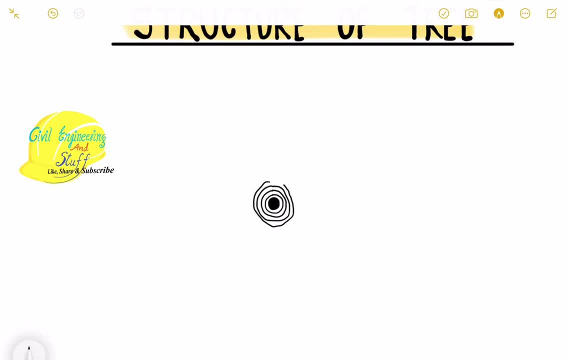 packed points, right. so when drawing this schematic, schematic diagram of the structure of tree, don't bother much about drawing a proper circle, right, because seldom you see a tree that is completely circular in shape. it has somewhat distorted shape, right. all trees have somewhat distorted shape, so don't worry about that. all trees have somewhat distorted shape, so don't. 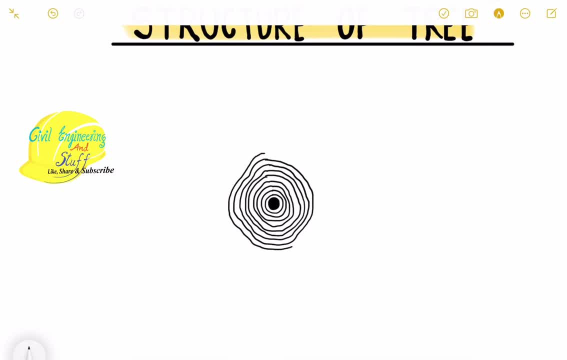 worry too much of drawing perfect circle. so we have inner rings that are closely packed, and after that we have outer rings that are somewhat placed at a further distance compared to that of inner rings, right, so we have these outer rings, and after the outer rings we have 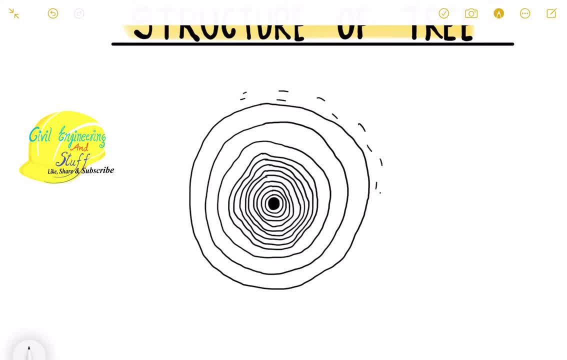 fibrous mass. we have fibrous mass and after that we have right. so let us discuss about each part. and we have some rays that emerge from pith and goes to the outer ring or the cambium layer that we are going to discuss just now. okay, so this is how the structure of the tree looks like, so let's discuss about each. 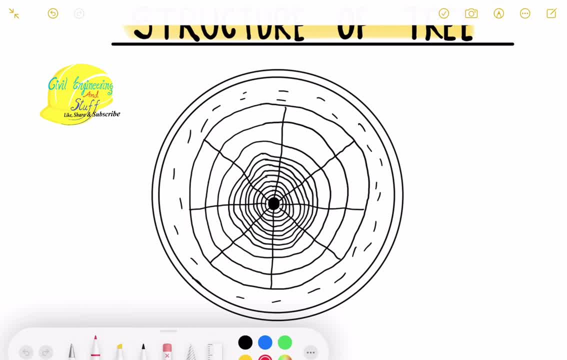 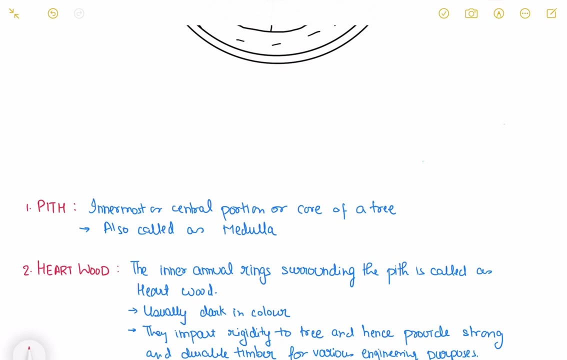 so in this the center point is called as pith or medulla. the center point is called as pith or medulla, right? so your pith is the innermost part of the tree, or the innermost portion or core of the tree, and it is also called as medulla. 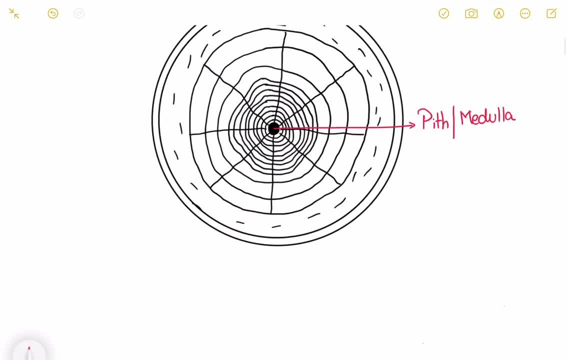 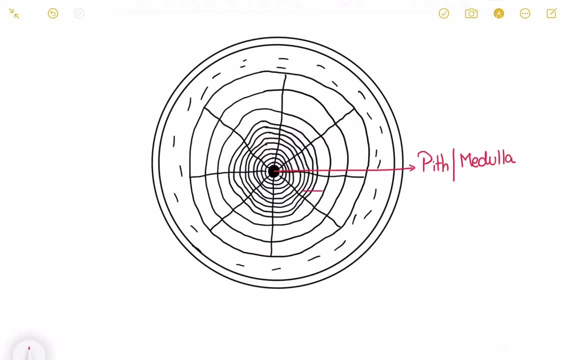 after this surrounding pith, we have the inner rings, these closely packed inner rings. these closely packed inner rings are called as heartwood, as we have seen in the image before that. these are closely packed right and are denser in color right. so your heartwood are the annual rings. 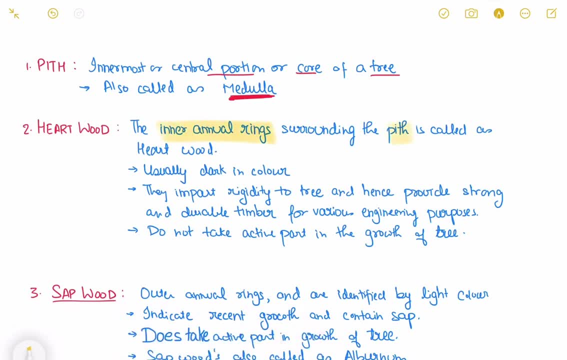 are the inner anul rings surrounded by surrounded the pith, and they are usually darker in color. they, that is, the heartwood, provides the rigidity to the tree. this means that the strength and durability of a tree comes because of the heartwood, right? so your heartwood is responsible for the rigidity that is. 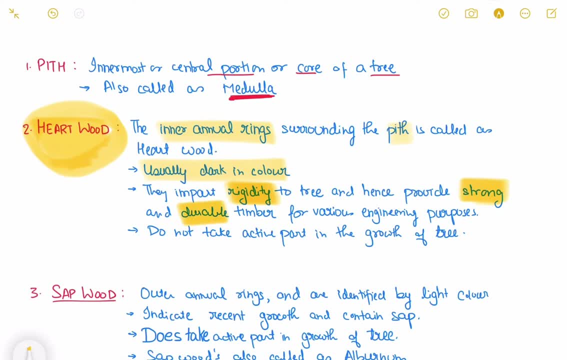 it makes the tree strong and durable, right. an important point that should be noted about hardwood is that they do not. they do not take active part in the growth of tree. right, they do not take active part in the growth of tree. they make the tree strong and durable, but they. 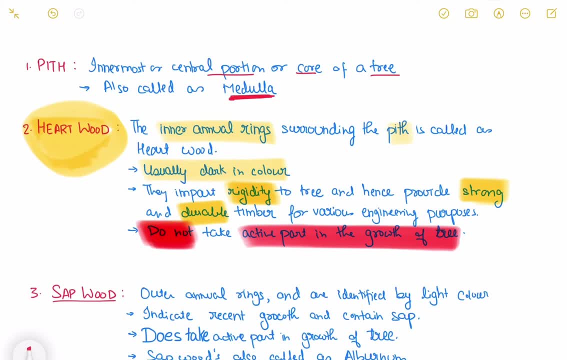 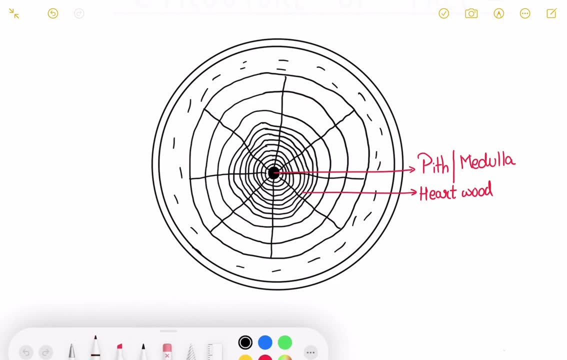 do not contribute much towards the growth of the tree. then, after this, we have some outer rings. we have some outer ring that are placed, compared to the hardwood tree, somewhat further distance right. so these outer rings are called as sap wood. the outer rings are called as sap wood. 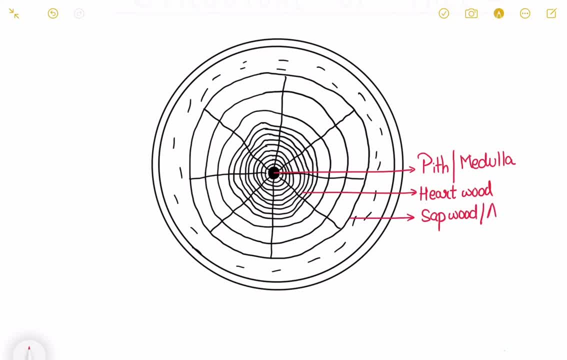 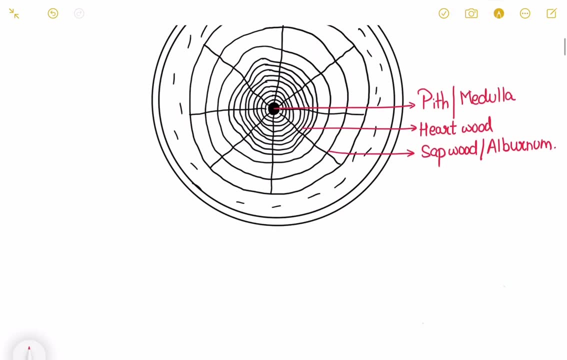 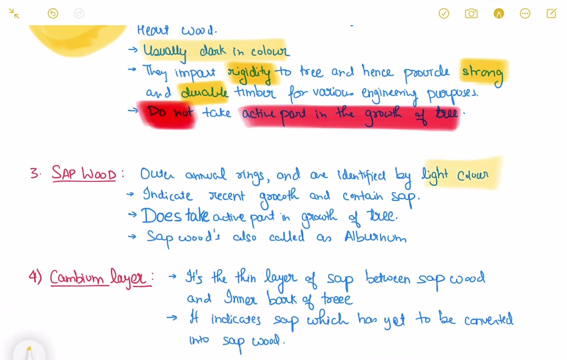 also called sap wood, called as alburum, also called as alburum. right, so these outer rings, these outer rings are called as sap, now is sapwood. the outer animal rings are identified by the light color as we have seen in the image before. they have comparatively. 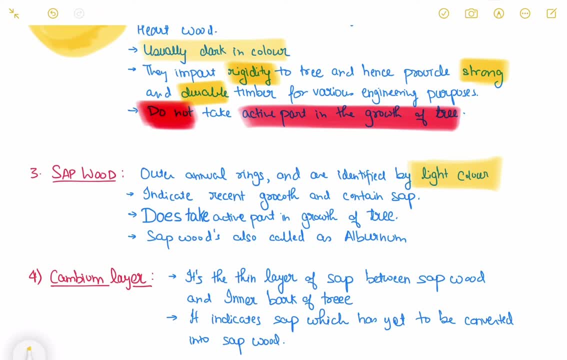 lighter color and these rings indicate the recent growth. right, these rings indicate the recent growth and they contain the sap, hence called the sapwood. now, these are the rings that takes the active part in the growth of tree right. so these rings, or the sapwood, take the active part in the growth of the tree. 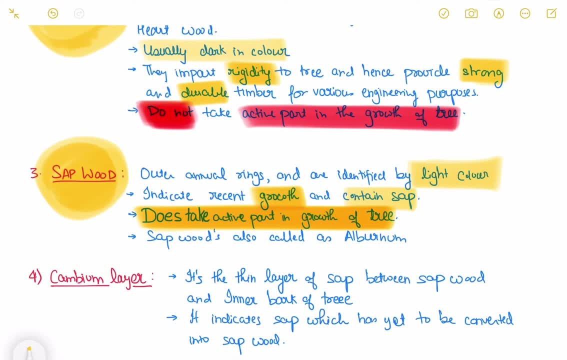 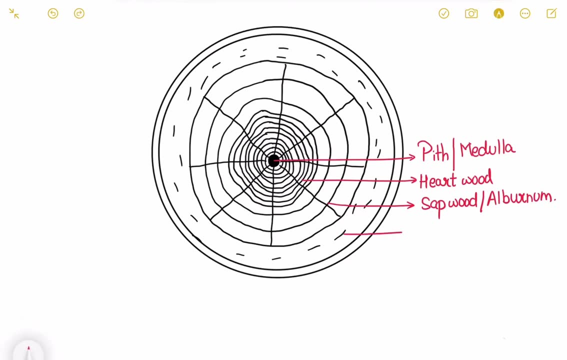 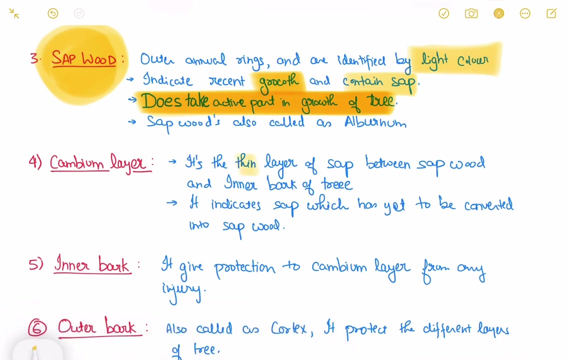 and contribute very much less to the growth of the tree, towards the strength and durability of the tree. right after outer ring we have as cambium layer. after outer ring or the sapwood, we have cambium layer and your cambium layer it is the thin layer that contain the sap. right it is the layer. 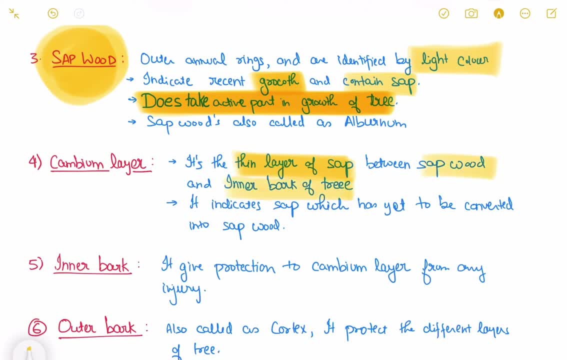 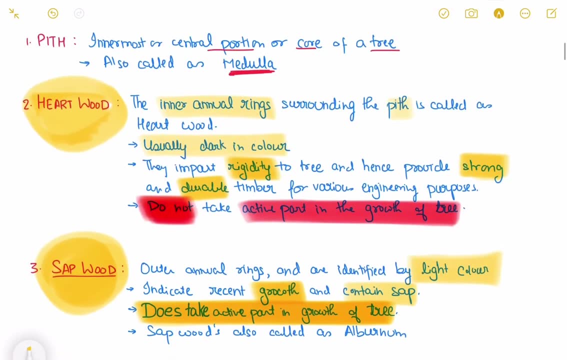 that contain the sap present between the sapwood and the inner bark of the tree and only the sap known obtained as sapwood, and the inner bark as lacking in the soil. the only sap known obtained as sapwood is awesome. this sap is yet to be converted. 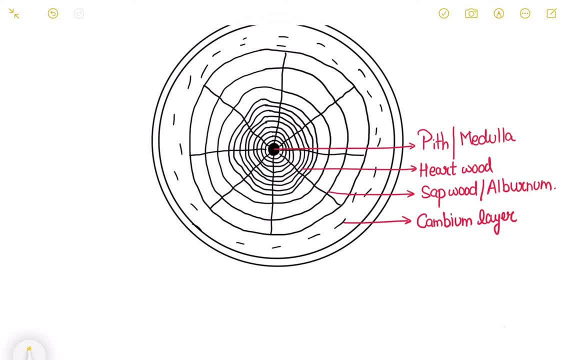 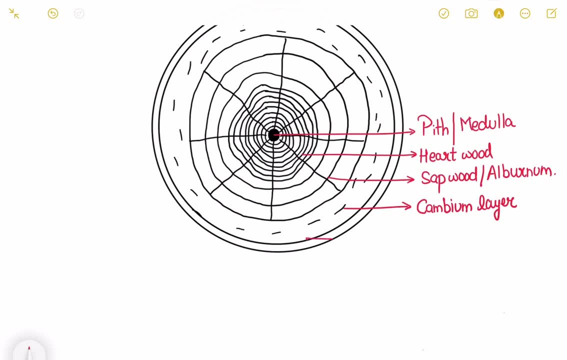 into sapwood right. so as the tree will get old, it will convert into sapwood, that is, it will start to form the outer animal rings. right after this we have the inner bark of the tree. this is called as inner bark of tree, esaoras petaflora sp. groomifolia daurers. 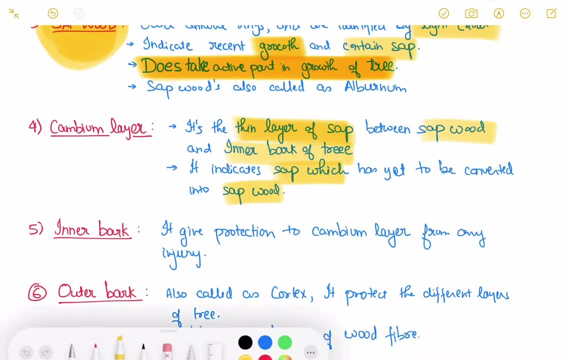 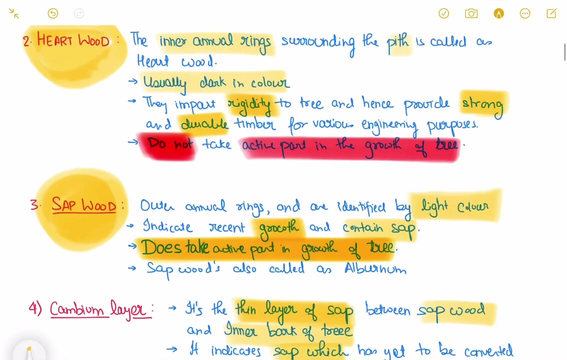 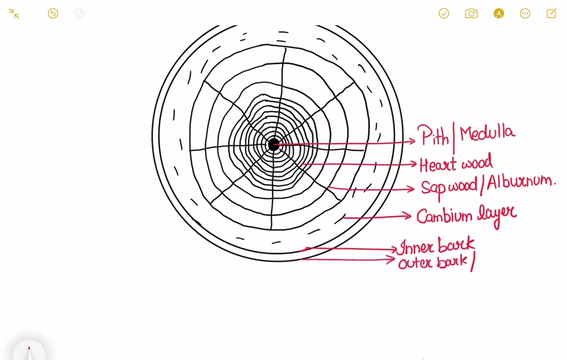 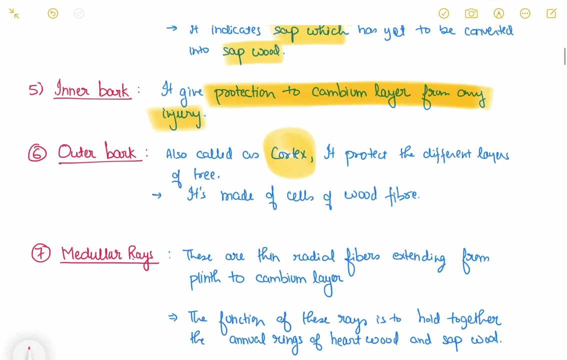 inner bark of the tree. it gives the protection to the cambium layer from any injury. it protects the cambium layer from any injury. and then we have outer bark, also called as cortex. so let me write down: I have the outer bark called as cortex. right, so a cortex, or the outer bark, protects. 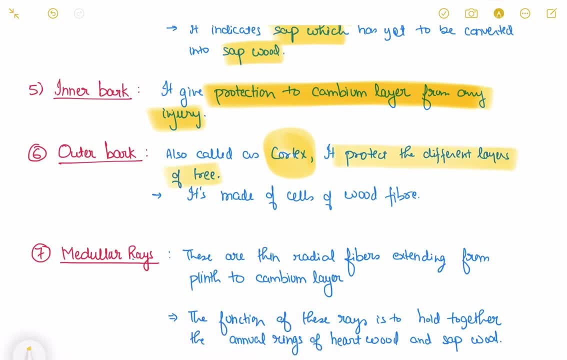 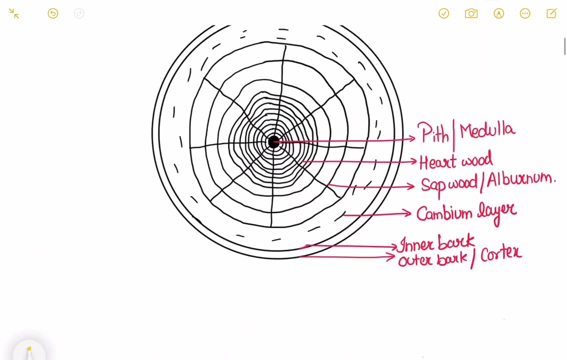 the whole of the assembly. it protects the whole of the assembly of the tree and is made up of cells of wood fiber. now, after this, we have we have these rays that are created from the outer bark. but we need to look at the outer bark. it is the outer bark or the outer bark of the tree. so we have these rays that. 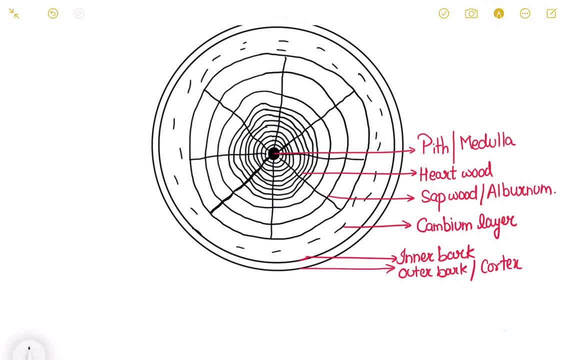 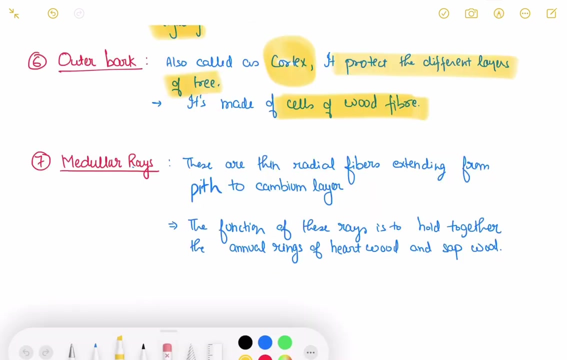 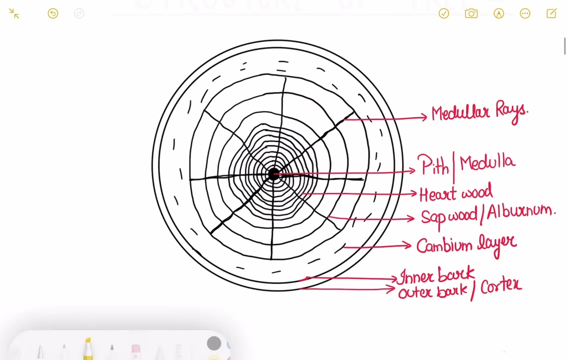 originate from the pith and goes towards the cambium layer at these rings, so these are called as medullar rays. so your medullar rays are the thin radial fibers that extend from pith to the cambium layer. they extend from pith to the cambium layer. right, they extend from.